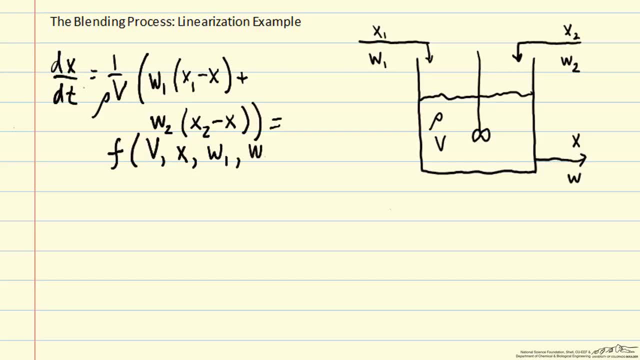 We also have inlet mass flow rates, w1 and w2.. And in this case we're going to assume that the mass fraction x is the mass fraction of the tank, That our density rho is constant. We're also going to assume that the inlet mass fractions x1 and x2 are constant. for this example, 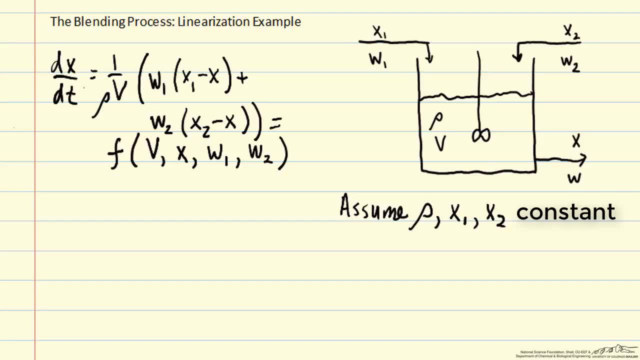 And now we're going to calculate the linearization of this nonlinear dynamic equation. For the left-hand side we'll substitute in deviation variables, So instead of x we'll have x bar the steady state value, plus x prime, the deviation from steady state. 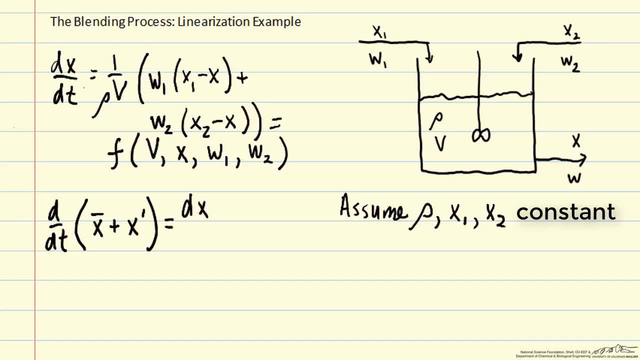 And because x bar is a constant, we can then simplify that to dx, prime, dt. So the deviation is time-varying but the steady state value is a constant. And then we're going to approximate the right-hand side by a first-order Taylor series approximation. 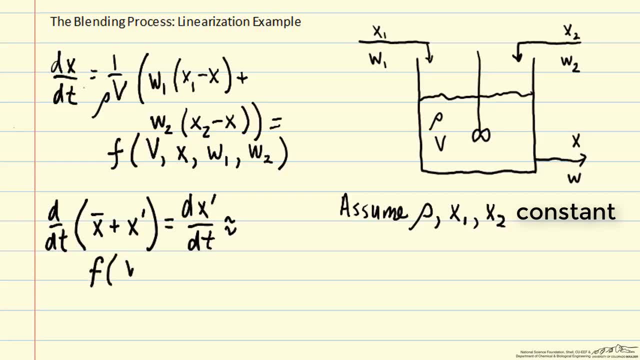 So we start off by evaluating f at the steady state And then we add on linear terms associated with each of the independent variables- And our first-order Taylor series is f, And then we add on linear terms associated with each of the independent variables. 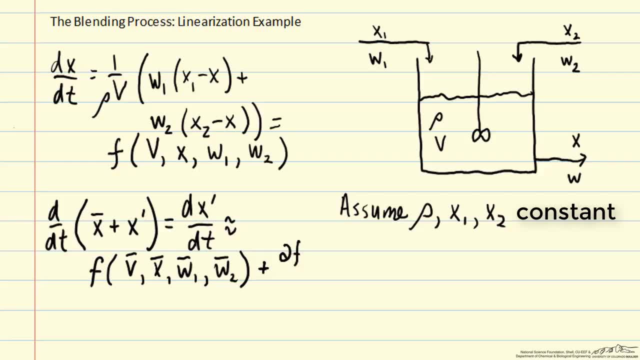 And then we add on linear terms associated with each of the independent variables. So we have df dv evaluated at steady state. We'll use ss for steady state Times v prime plus df dx evaluated at steady state times s prime, plus df dw1 evaluated at steady state times w1 prime. 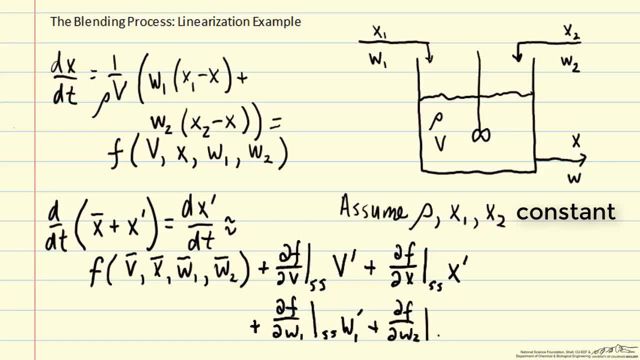 Plus df, w2, evaluated at steady state times, w2 prime. So one thing to notice here is that when we evaluate the derivative of f with respect to each of these independent variables, we are evaluating at the steady state value And those are going to be constant values. 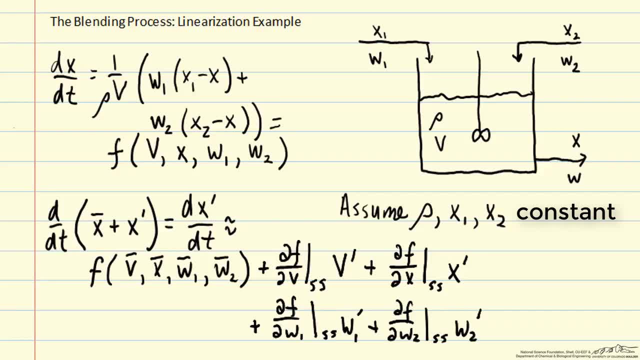 So the only time-varying quantities in this new model are going to be associated with the deviation variables, And those all enter linearly. So that's the left-hand side. The reason that this model is going to be linear is because we're using only a first-order Taylor series approximation. 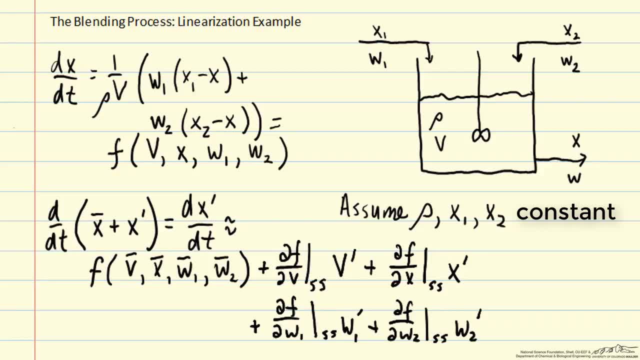 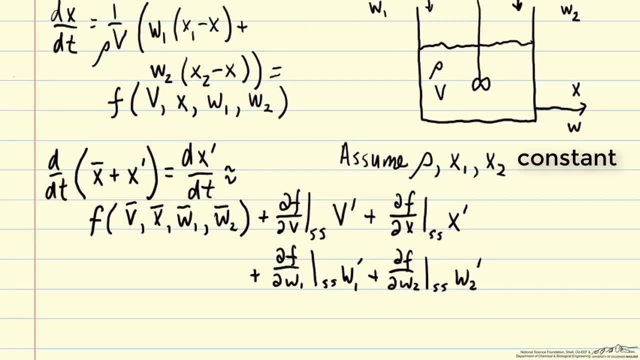 If we wanted it to be more accurate, we could include higher-order terms, but then we would be back to having a nonlinear model. Now let's go ahead and plug in our function f and its derivatives into this approximate linear model. First we need to evaluate this function at its steady-state value. but the function is just the time derivative of x. 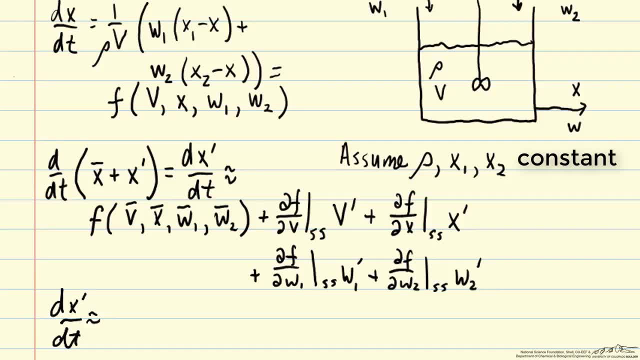 and at steady-state we can plug in 0, dx, dt equals 0, and the bar variables on the right-hand side, and so this term is always going to be 0 for any linearization around steady-state. so that's very convenient. 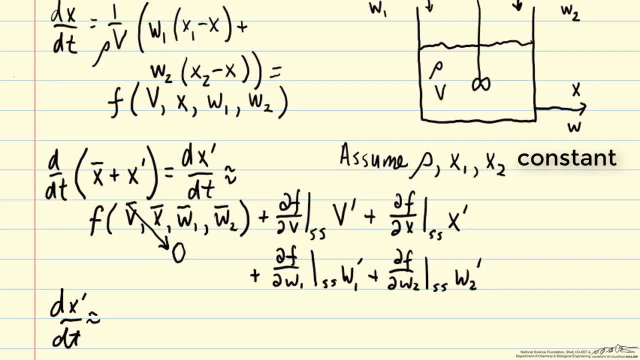 We can always cross off that term as long as we're linearizing around steady-state. But we do need to go ahead and evaluate these derivatives Now. the first derivative is going to be the messiest because we have 1 over v and in our differential equation we'll go ahead and evaluate the derivative of f with respect to v at steady-state. 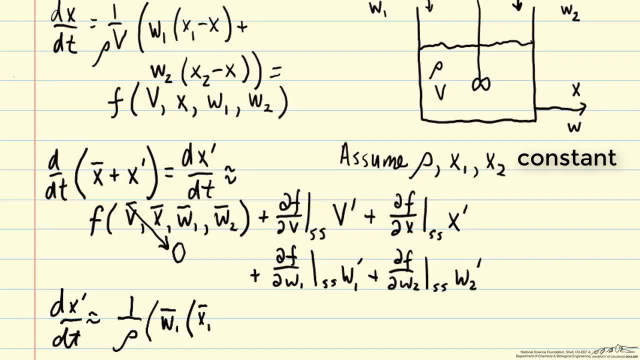 So we're basically just going to rewrite all these other terms that we're going to hold at their constant value for this derivative, and then we're going to need to take the derivative of 1 over v, So we're going to get minus 1 v to the minus 2, and we're going to evaluate that again at the bar value. 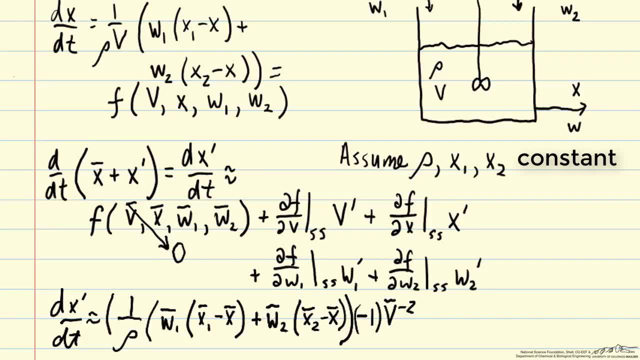 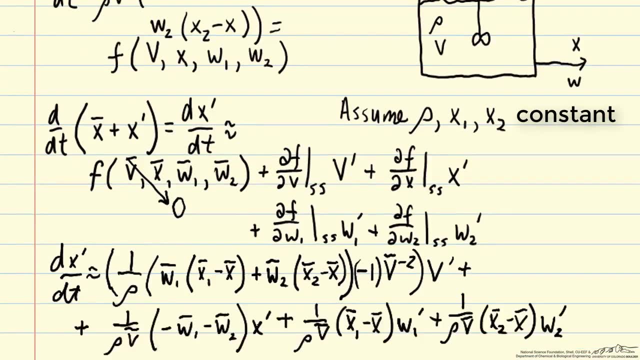 and then we're going to multiply this entire derivative df, dv by v' So that is our first term. We need to do that three more times, but fortunately the function is not as complicated in order to do that. So that is the linearization for any arbitrary steady-state of the system. but let's plug in some numbers. 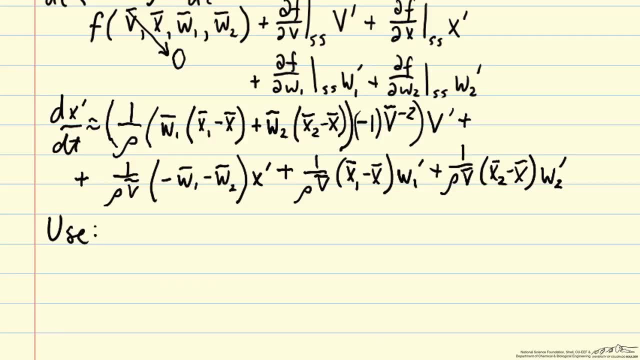 So we'll use the same values That we had used previously, And from these steady-state inlet conditions we can then calculate the steady-state outlet conditions. So w-bar is just the sum of the two inlet streams, So that's 4 kilograms per second.